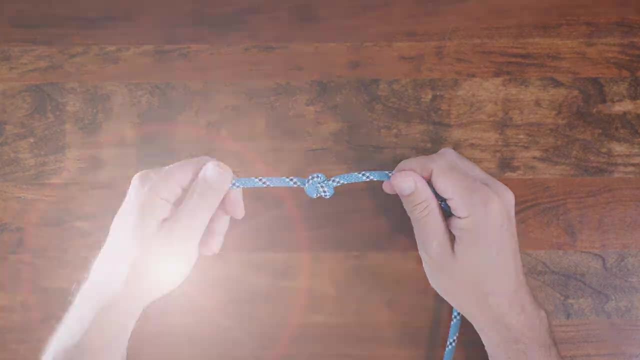 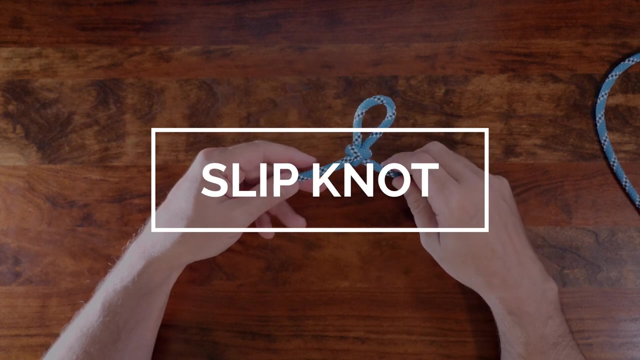 to do is pull on both ends equally to tighten the knot. Second on our list is the slip knot. The slip knot also belongs to the category of knots known as the overhand knot. The overhand knot is a knot known as stopper knots. There are many other stopper knots you can learn. I'll add a link to the. 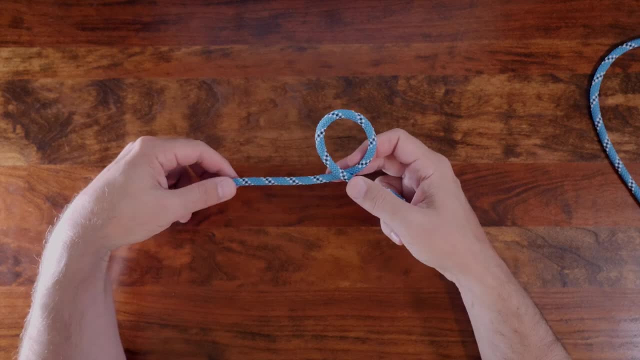 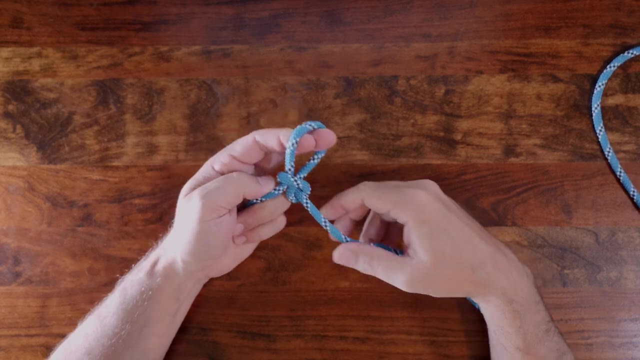 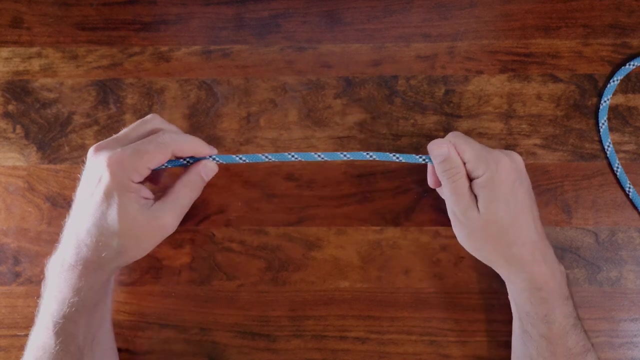 best nine stopper knots. in the description You'll recognize the basic structure of a slip knot with its similarities to the overhand knot. So the slip knot is a stopper knot which can be easily undone by pulling the tail end. Okay, so now let's have a look at how to tie the slip knot. So to tie the slip knot, first make a. 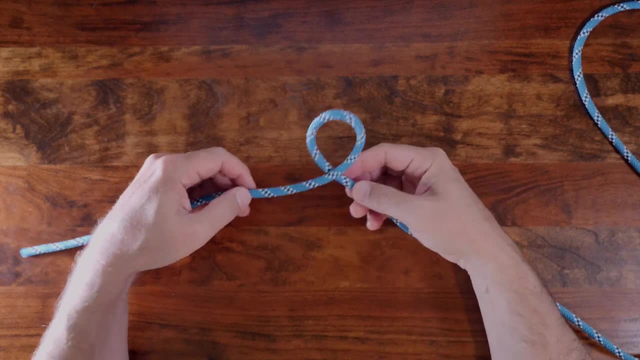 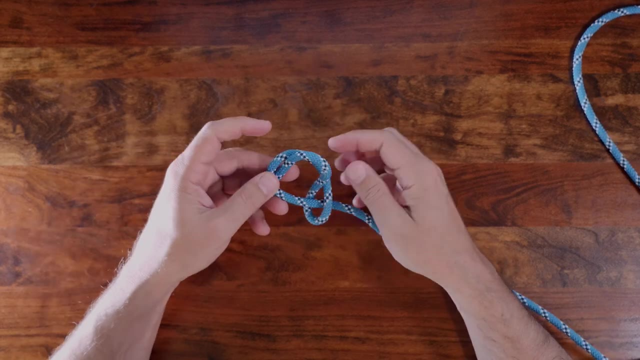 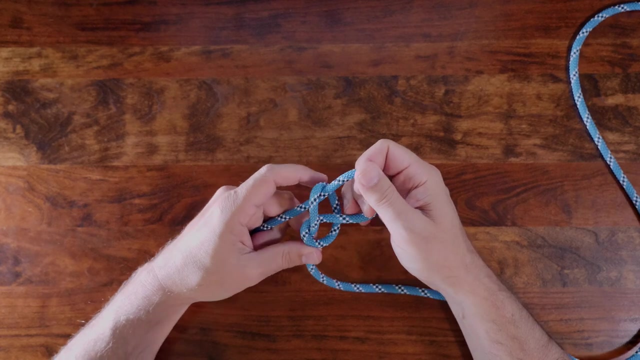 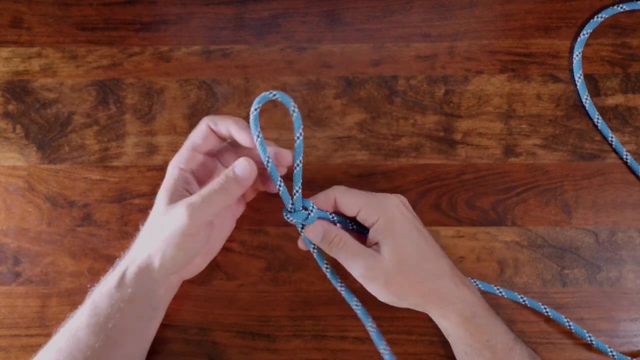 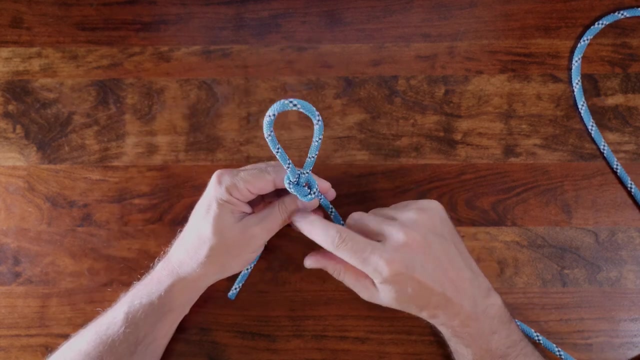 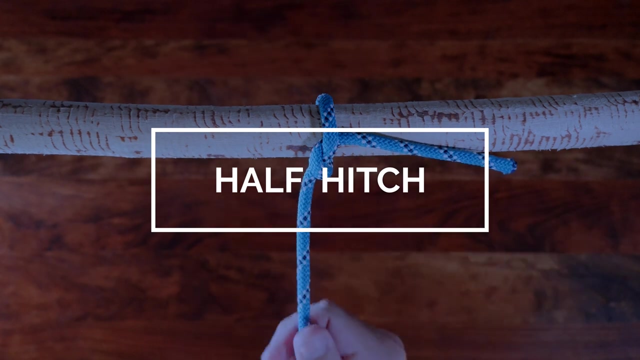 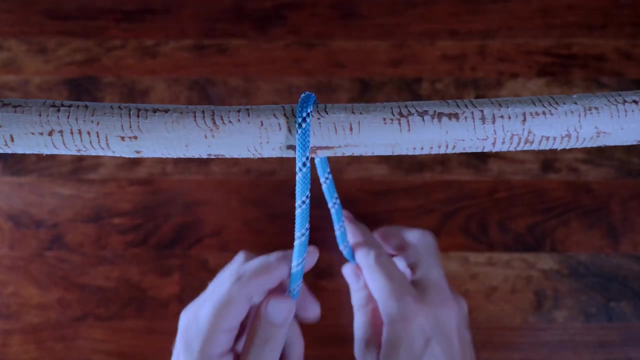 loop in the rope, Then pass a small bite through the loop, Finish it off by snugging it up tight. Next up in our list of the eight knots everyone should know is the half hitch, Another knot that owes its foundation to the overhand knot. you'll recognize the similarities. 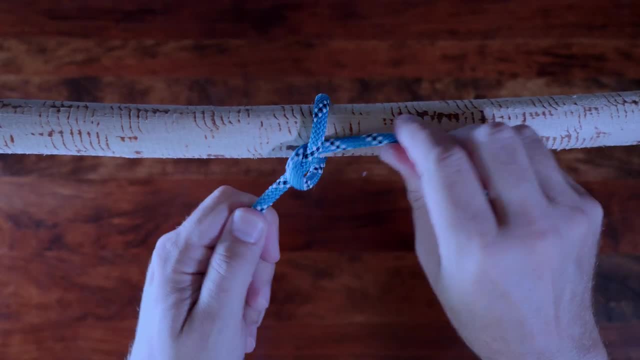 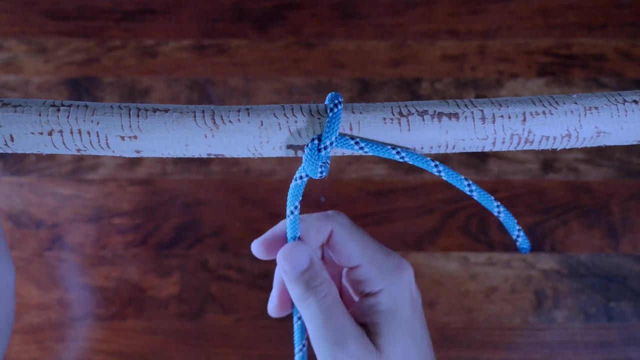 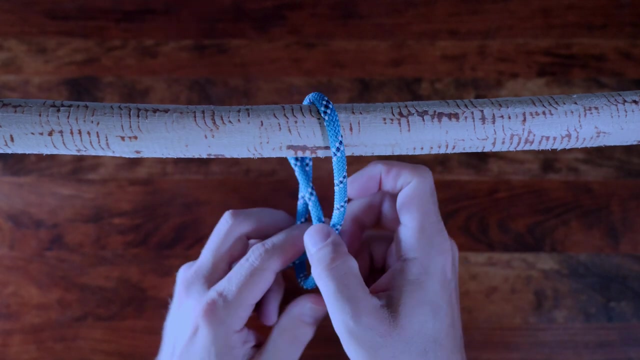 The half hitch is the first hitch knot we're including in the eight knots everyone should know. Similar to the overhand knot, the half hitch is a foundation of many other hitch knots that are available to learn, Although the half hitch is known as being unreliable and that it can slip. 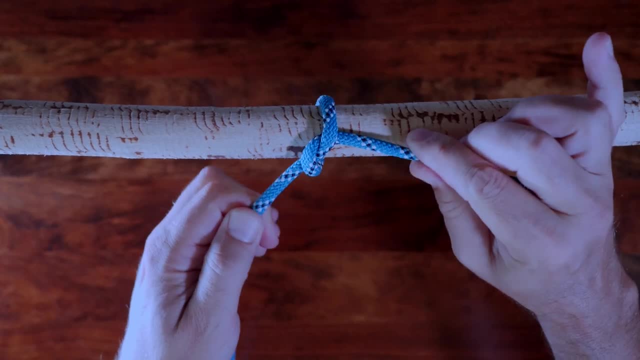 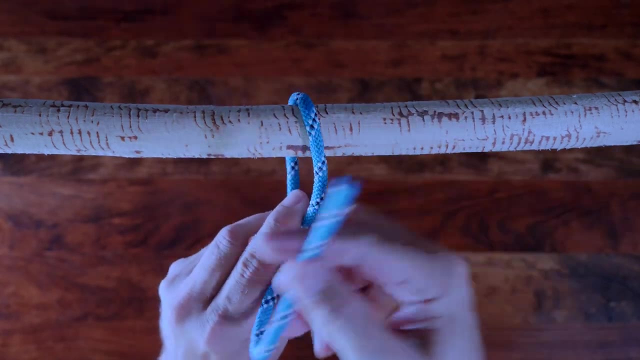 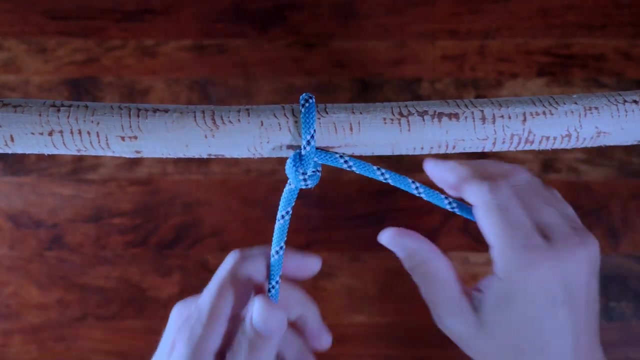 and become undone. its importance as a foundation knot is why it made our list. So to tie a half hitch, all you need to do is pass the working end of a rope around an object and then tie an overhand knot. You can see as I pull on the line the half hitch tends to slip. 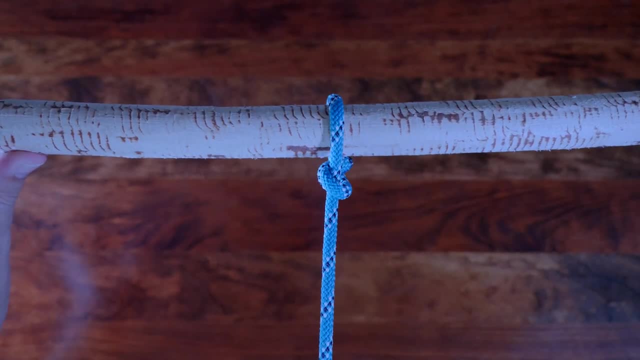 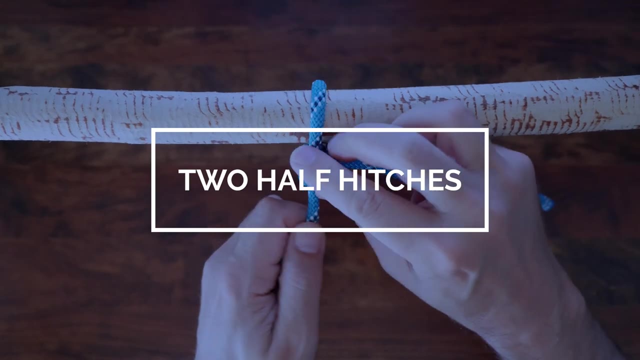 It's very easy to make the half hitch a more reliable knot. All you need to do is double it up and make it two half hitches knot. Continuing to build on the knot tying skills we've already developed and still working with the basic overhand knot. we're now improving on the 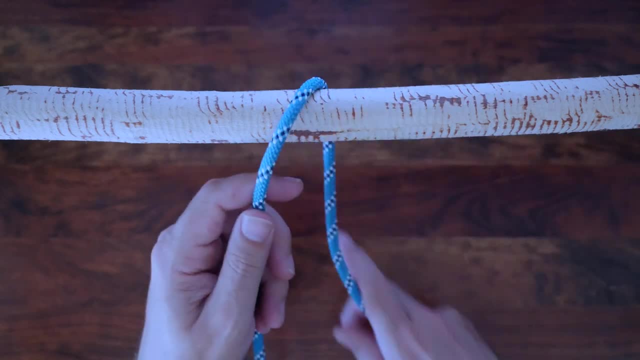 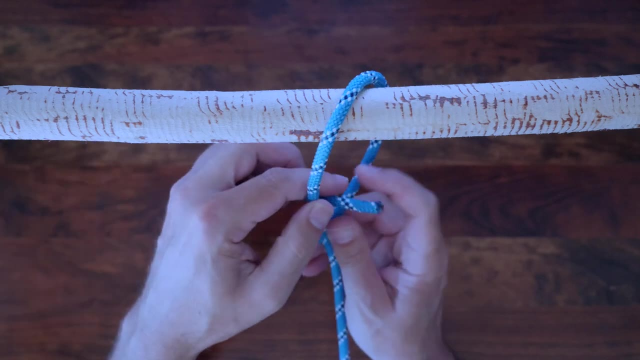 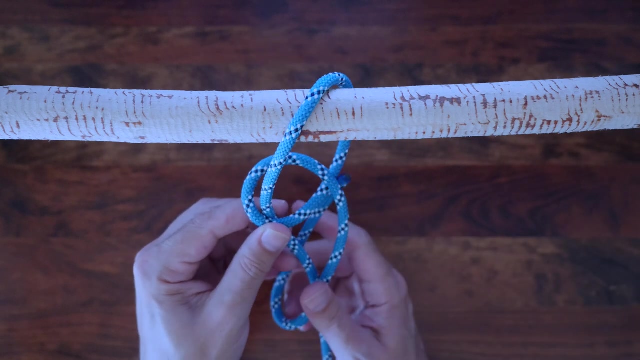 half hitch, making it more secure and reliable with the two half hitches knot. Sometimes the two half knot is called a clove hitch over itself or a double half hitch. It's sometimes also called a full hitch. The two half hitches is an overhand knot tied around. 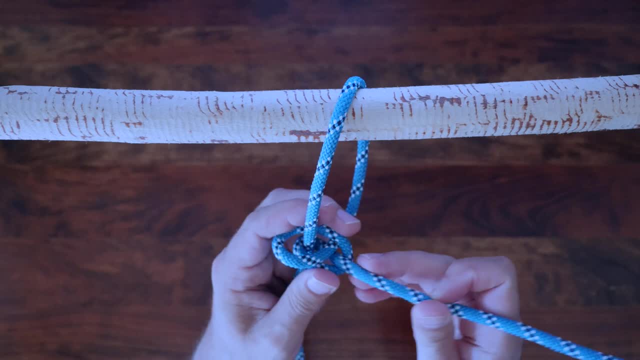 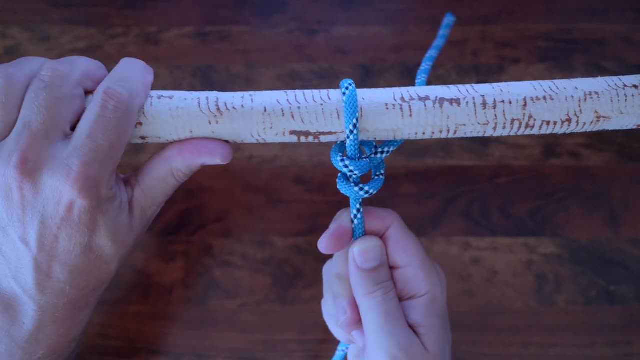 a post followed by another half hitch. So when tying the two half hitches, knot always tie the half hitches in the same direction. So if you start the first half hitch with the tail passing away from you above the rope, then do the same with. 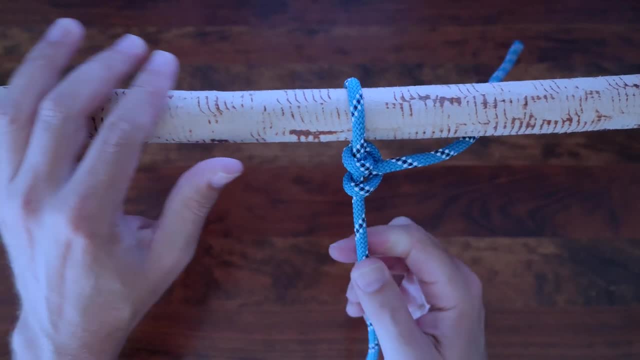 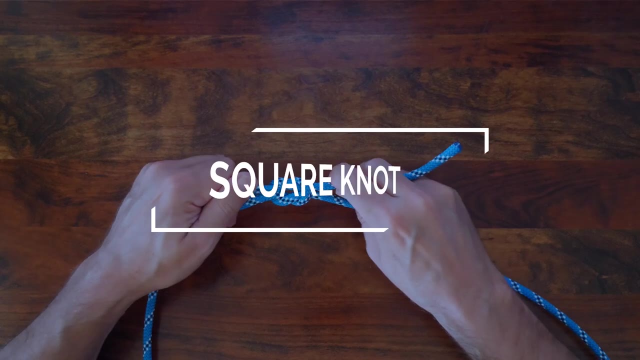 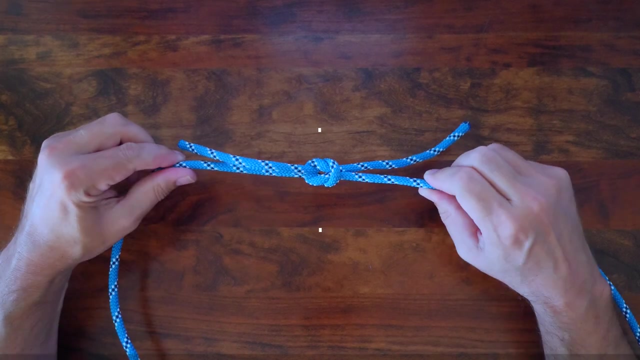 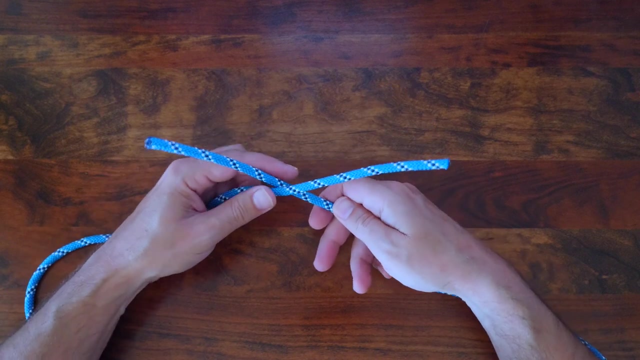 the next. We're halfway through our list of eight knots everyone should know. and next on our list is the square knot. So the square knot is also known as the reef knot or the Hercules knot, and it's a binding knot, but it can also be used as 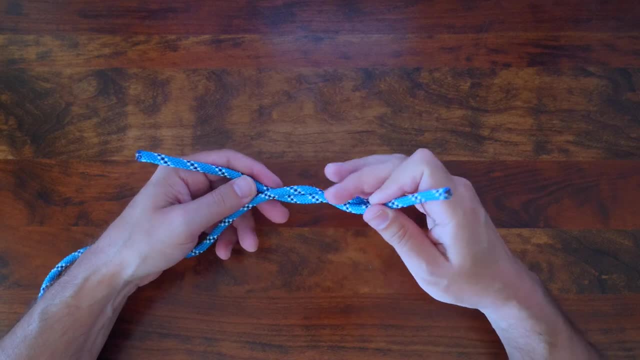 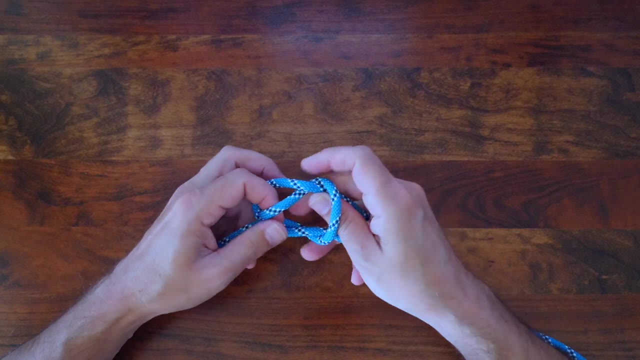 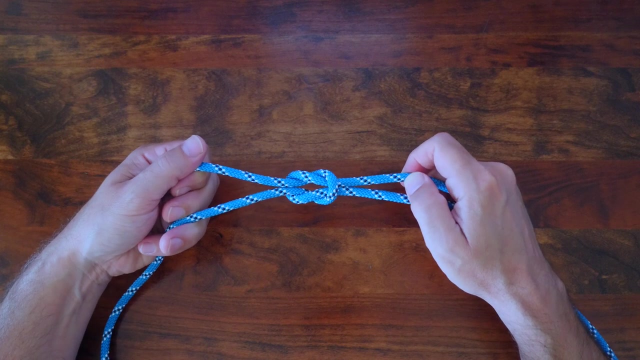 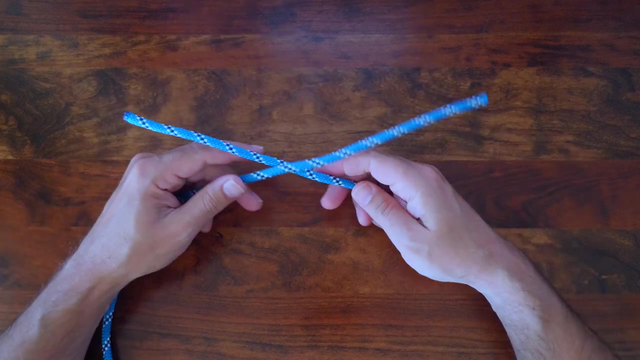 a bend. A bend is a category of knot that is used to join two different ropes together with a knot. The square knot is created by tying a left overhand knot, followed by a right overhand knot. Now let's look at how to tie the square knot. Begin by overlaying the two lines, then 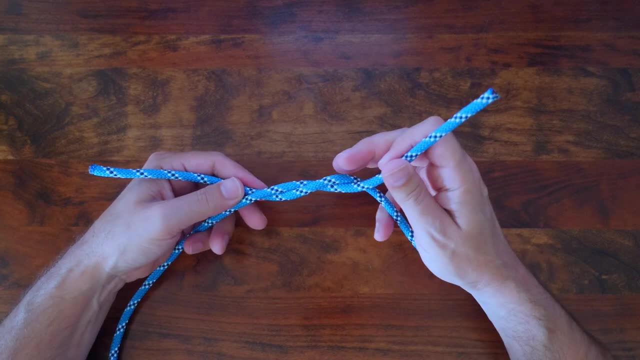 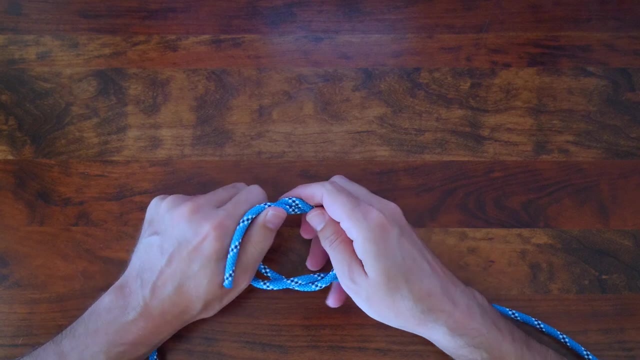 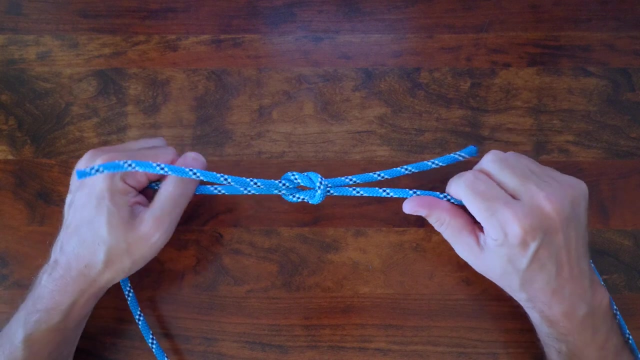 pass the working end once around the other line and bring the ends to the top. Then pass the working end once more around the other line in the opposite direction. An easy way to remember how to tie the square knot is to remember left over, right, right. 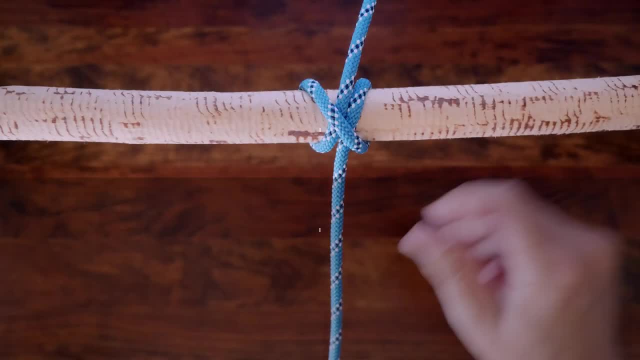 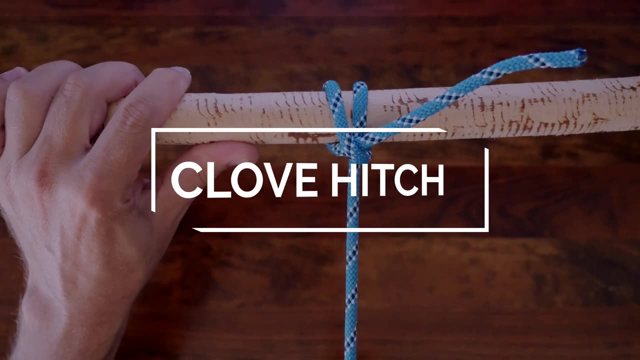 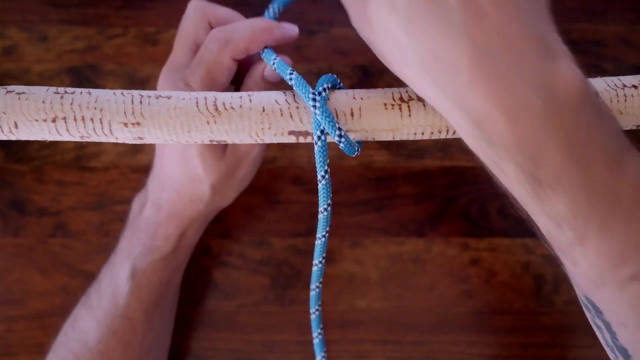 over left when forming the overhands. Let's keep moving as we work through the eight knots everyone should know. Next up is the clove hitch. The clove hitch is another great knot. The clove hitch, as one would assume by its name, is another hitch knot, and it's often 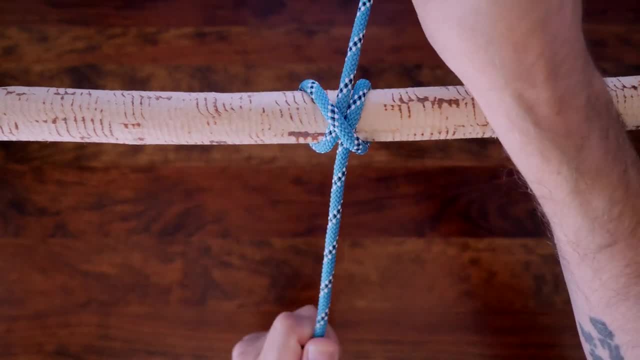 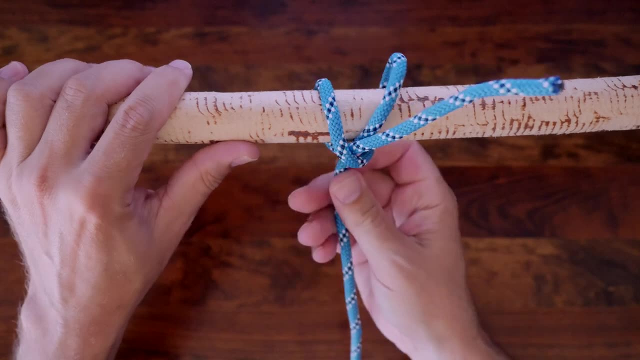 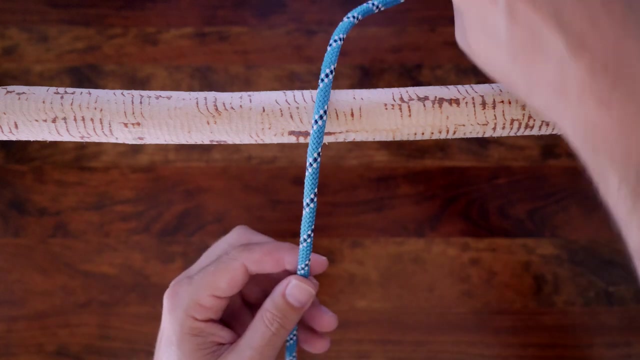 considered one of the top three knots that you should learn. The clove hitch is a hitch knot and it's often used as the starting knot when you begin to tie lashing. It's a popular hitch knot because it's easy to tie and it's also very easy to untie. 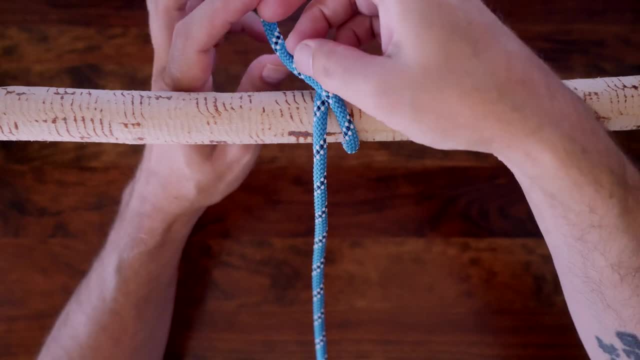 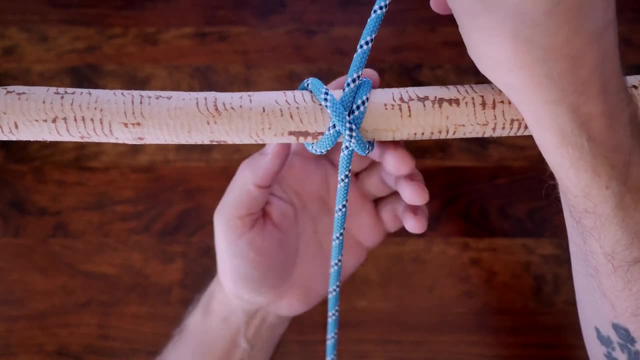 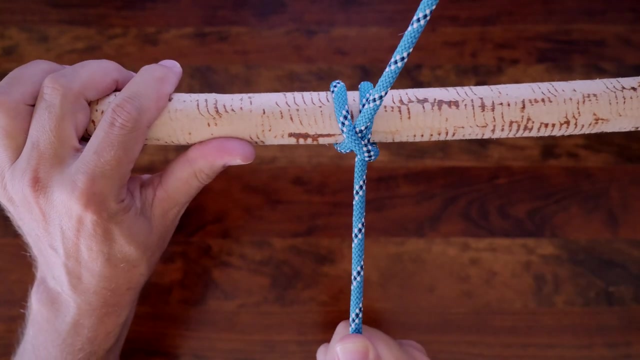 even after it's had a substantial weight. A bit of caution should be taken when using the clove hitch, because it can come undone easily, especially when constant pressure isn't being put on the line. I'm going to show you two ways to tie the clove hitch. 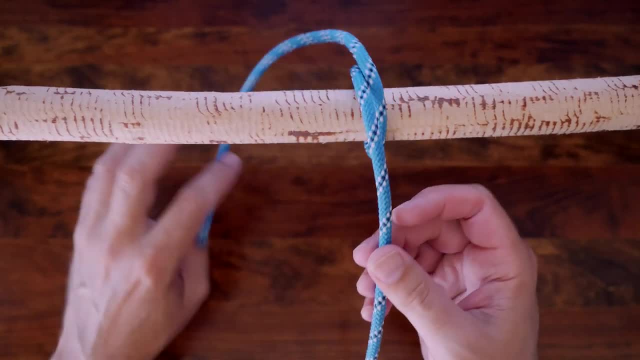 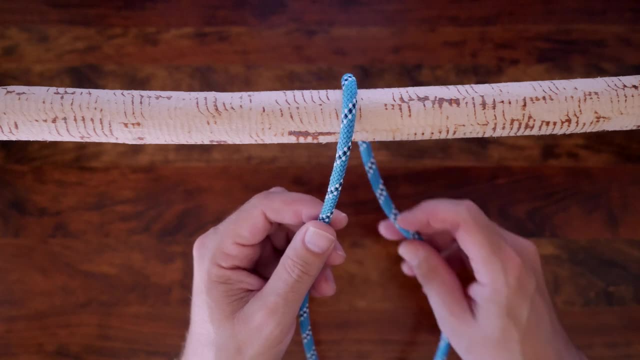 The first way to tie the clove hitch is used when you don't have an open end on your anchor point. So let's have a look at how to tie the clove hitch. Begin by passing your line around your anchor point, then cross over your line and around. 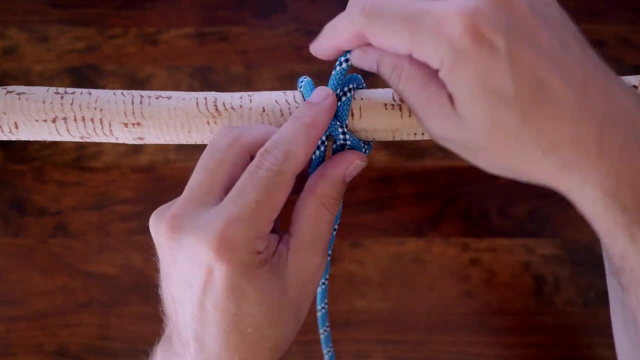 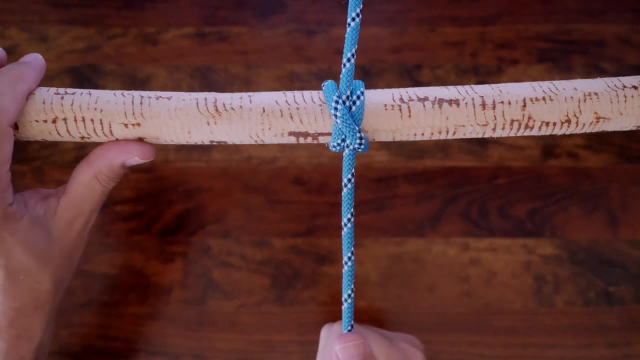 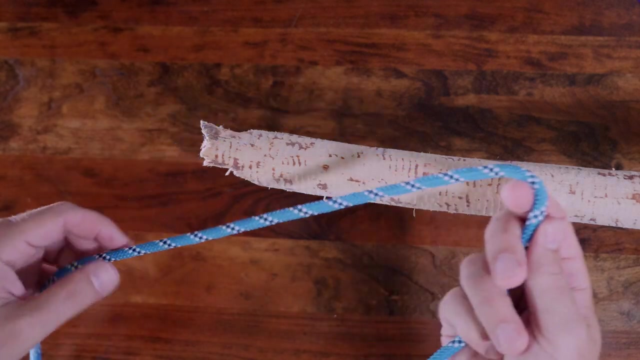 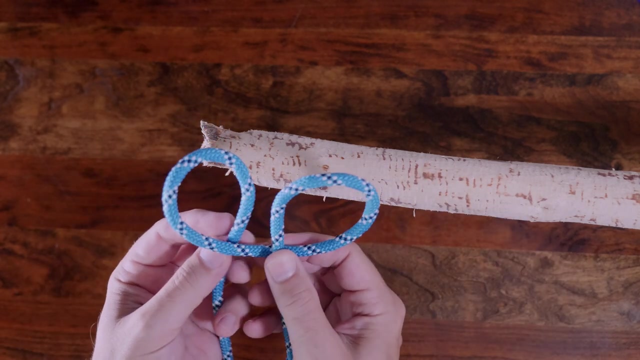 your anchor point again. Then slip your working end underneath your last wrap and from there pull it tight. The next way to tie a clove hitch is if your anchor point has an open end. Tying the clove hitch this way simply make a loop and then another loop and then place. 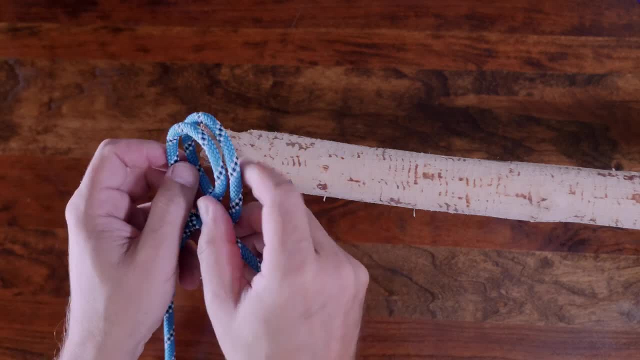 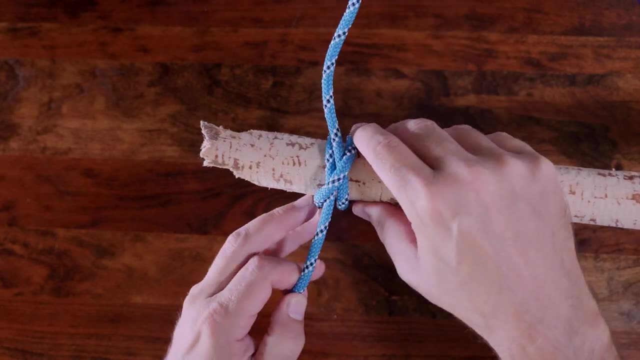 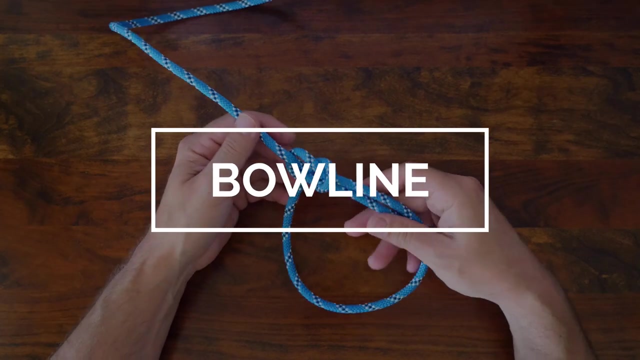 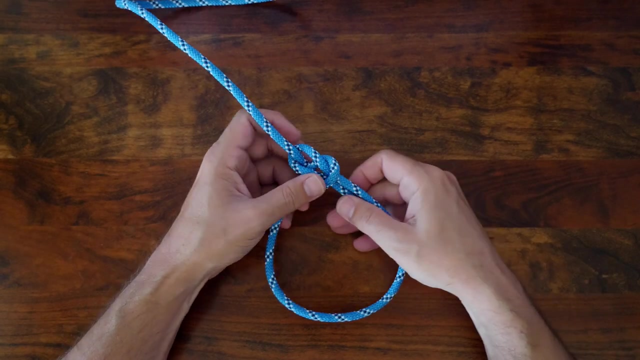 the second loop behind the first loop and then slide the loops over your anchor point And then pull it tight. Number seven in our list of eight knots everyone should know is the bowline, Often referred to as the king of knots due to its importance. the bowline knot is an 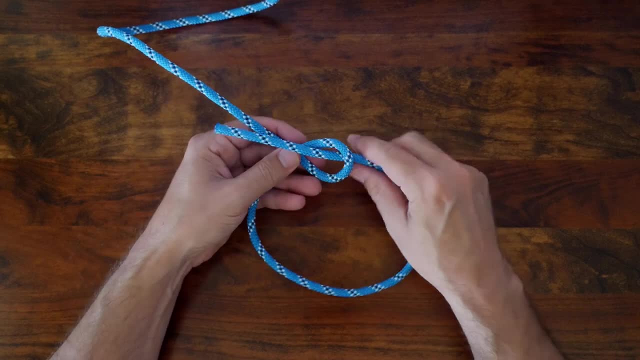 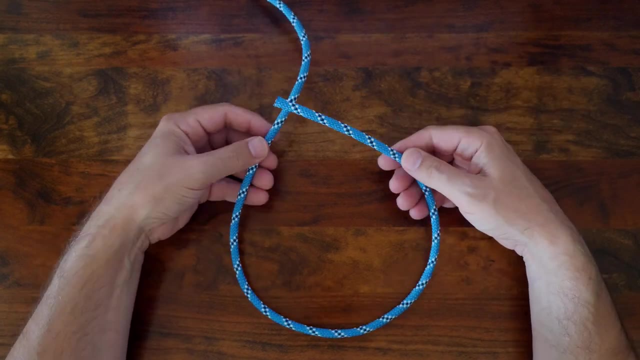 easy-to-learn way to tie a fixed loop at the end of a working line. Most importantly, it's easy to untie even after being subjected to a heavy load. So let's have a look at how to tie the bowline knot. 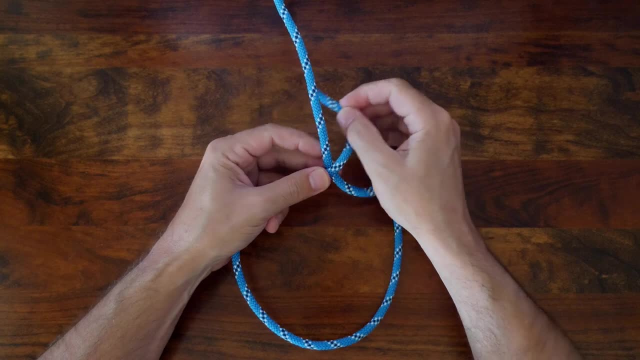 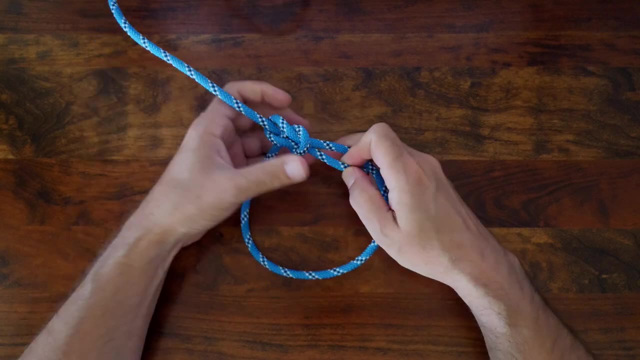 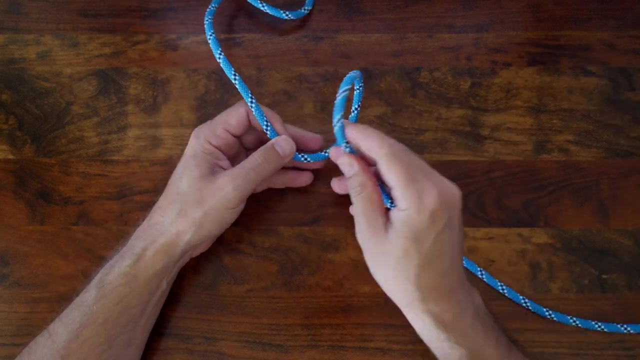 There are a few different ways to tie the bowline, but most people know the little story of the rabbit jumping up out of its hole, running around the tree and then back down the hole again. So the first step is to create a loop by twisting your working line. 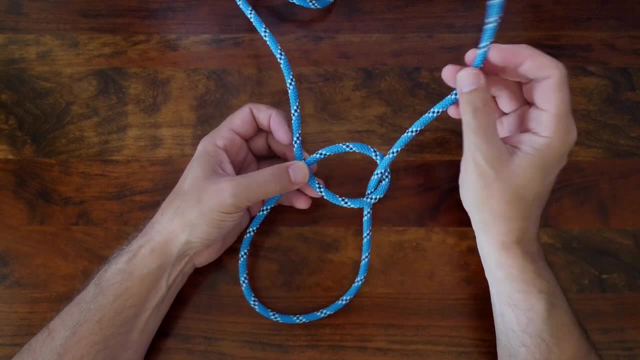 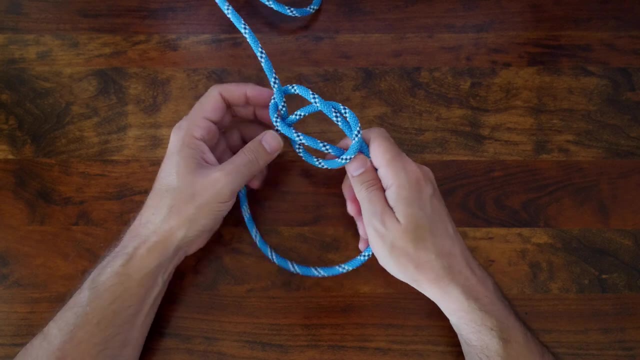 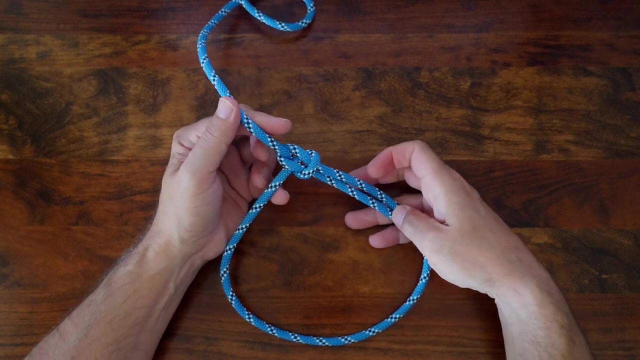 From there, take your working end and feed it up through the loop and then around the standing line and then back down through the loop. A properly formed bowline should have the working end on the inside of your bowline loop when it's finished.